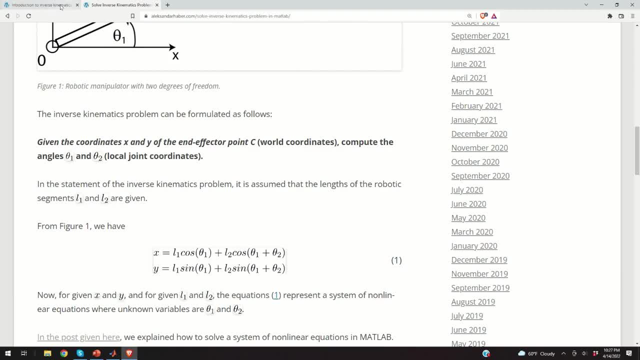 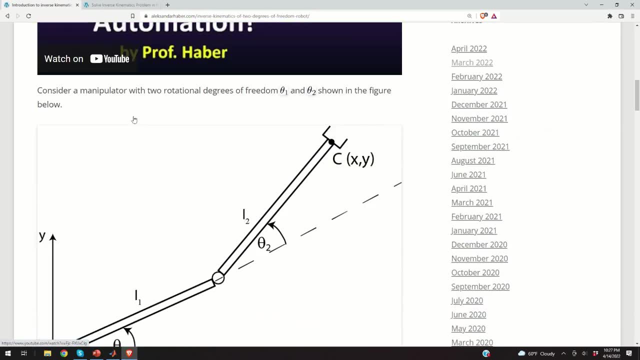 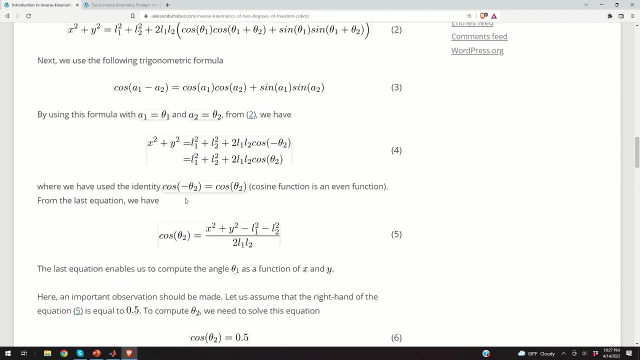 on how to derive these two equations. you can watch my previous video and you can read the tutorial that I made that's given over here. In this particular tutorial, I explained how to derive these two equations and how to solve them analytically for θ2 and θ1.. 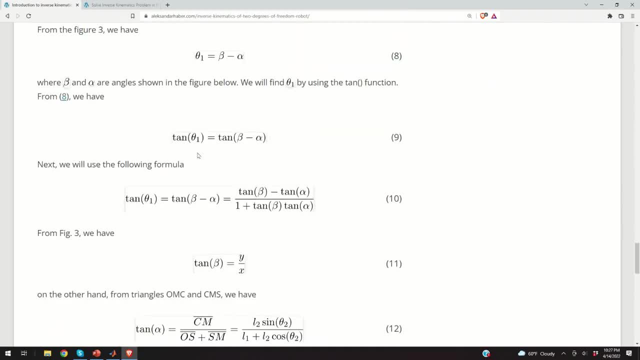 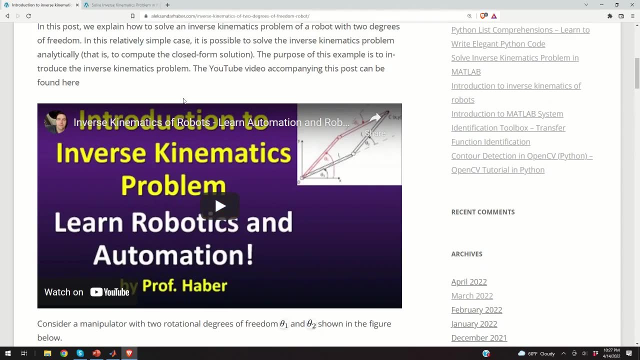 In the interest of the brevity of this video, I will not explain this procedure. If you want to refresh your knowledge or if you want to learn how to derive analytical solutions to inverse kinematics problem, please watch this video. Thank you very much. 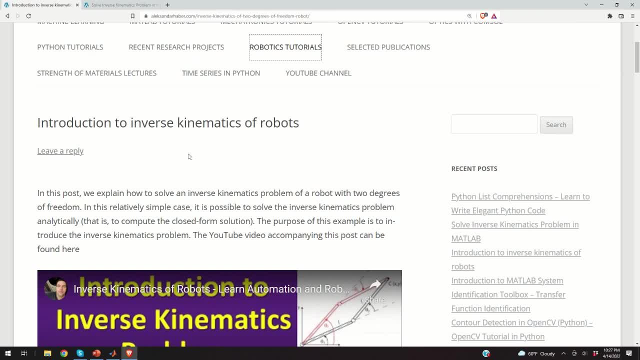 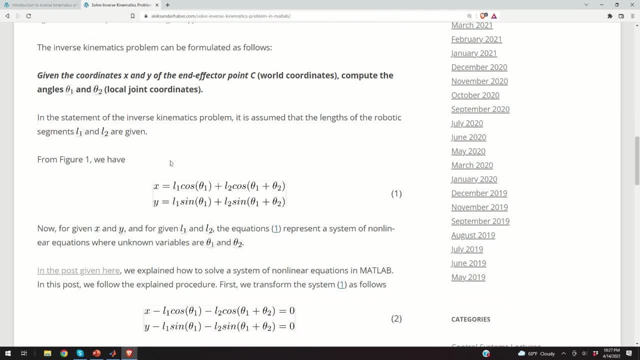 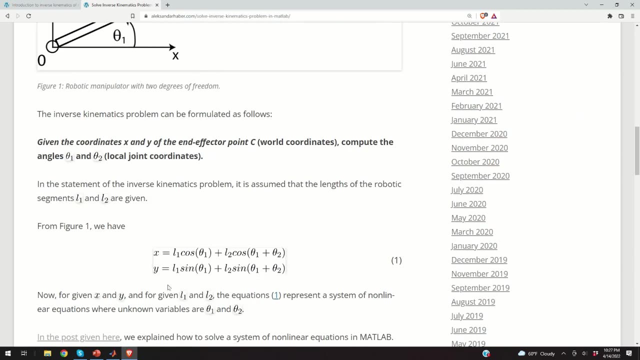 Thanks for watching. So let us back to our original problem. So, having these two equations that relate x and y, with the angles θ1 and θ2, I want to solve these equations. For this specific case, we can solve it analytically and this is explained in our previous video. however, 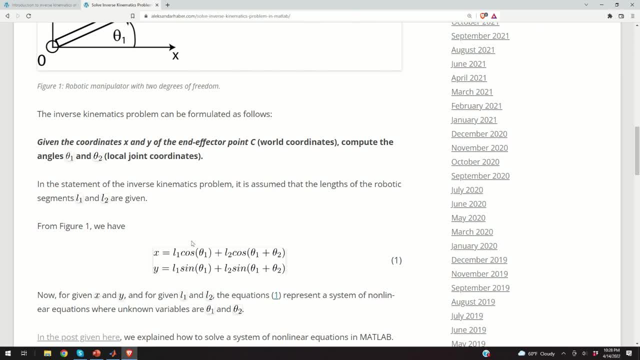 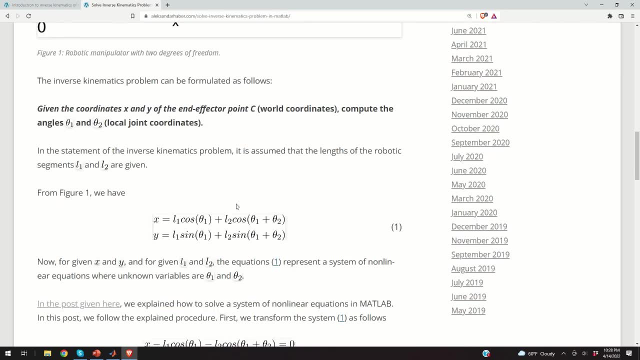 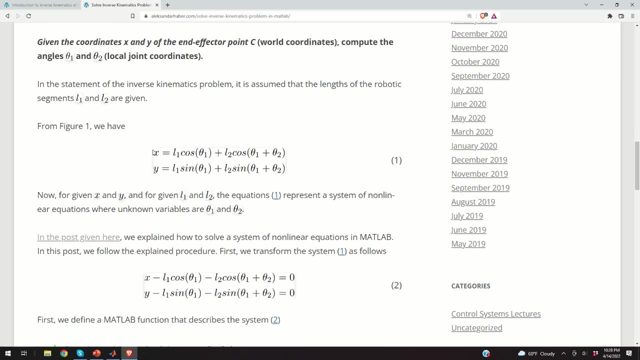 for more complex cases and robotic systems, which has more complex configurations and more degrees of freedom. it is challenging to solve these equations analytically. consequently, we have to solve the equations numerically. in this video, I will use MATLAB to solve these two equations. however, you can generalize this, this procedure and you. 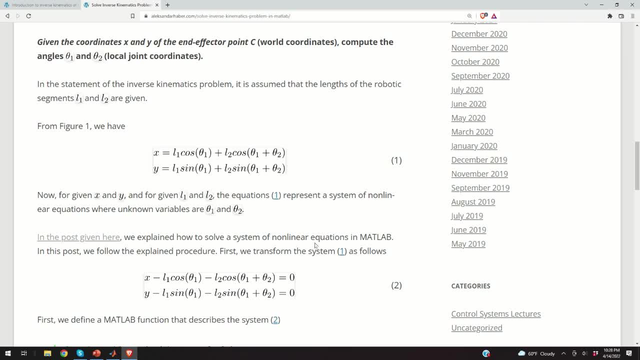 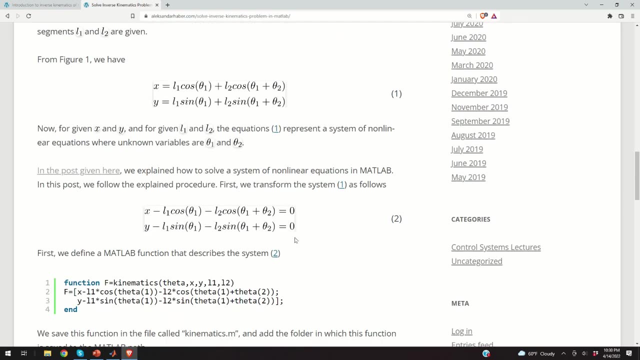 can write your own code in Python or C in order to solve these two equations for theta 1 and theta 2. the first step in solving this system of nonlinear equations for theta 1 and theta 2 is to write it in the so-called canonical form. 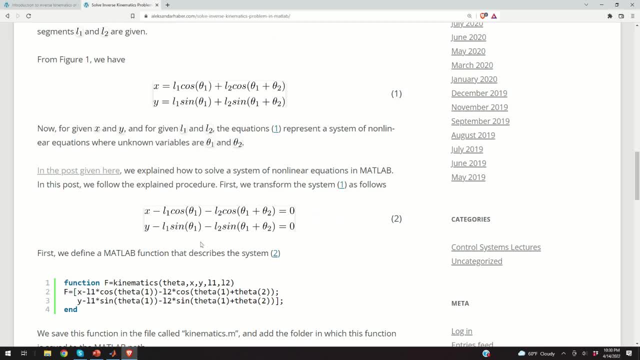 the canonical form is given by the equation 2, so you take all the terms on the right hand side and you write them on the left hand side with the corresponding minus signs, and on the right hand side you will leave zeros. once we have the system in this form, we can: 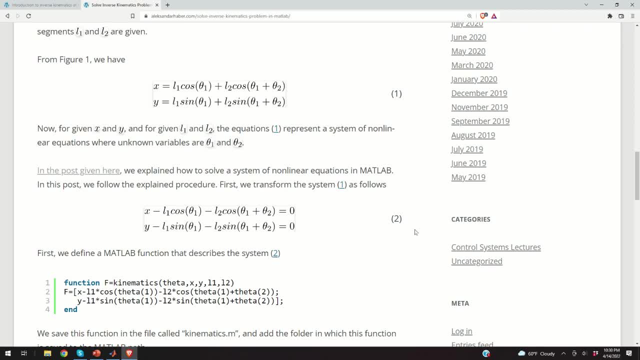 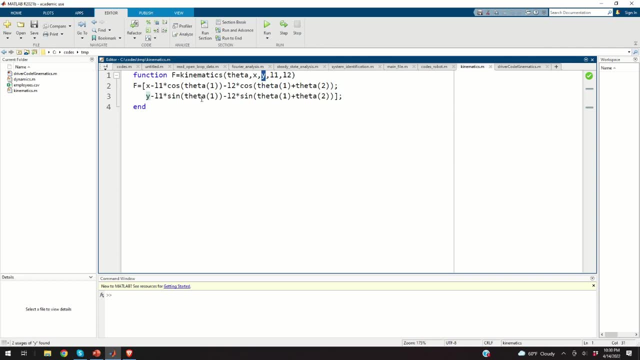 easily translate these two equations to MATLAB. so let's see how to do that. okay, so the first step is to write a function that will give the left hand side of the equation. this function will take theta as an argument. this will be a vector, and the first entry will be theta 1. the second entry will be theta 2. then we 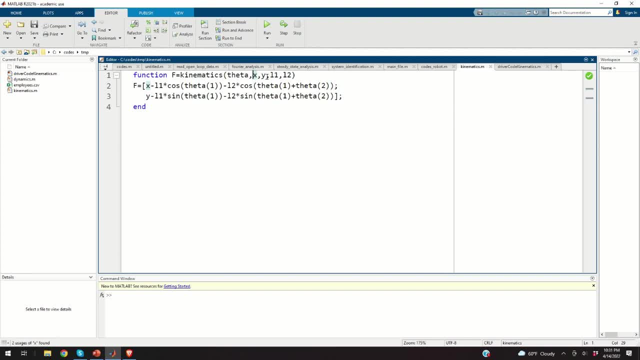 need to provide additional arguments, and these arguments are: X, Y, lengths of the segments l1 and the length of the segment l2. so, for the given theta, given X, Y, l1 and l2, this function will return the value of the left hand side. this would be a vector, for example. the function will return the value of the left hand side. this would be a vector, for example, the. 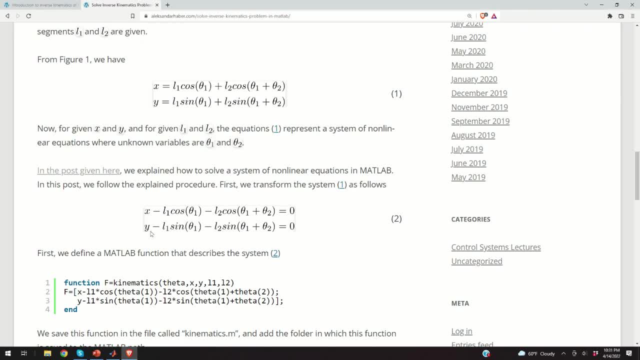 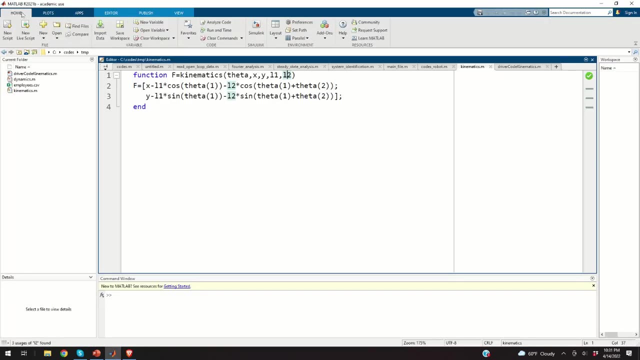 first entry can be 0.1. the second entry can be 0.2, if the equations are correctly solved, that is, if we know theta 1 and theta 2 accurately, the left hand side is 0. now what you need to do? you need to save this function in. 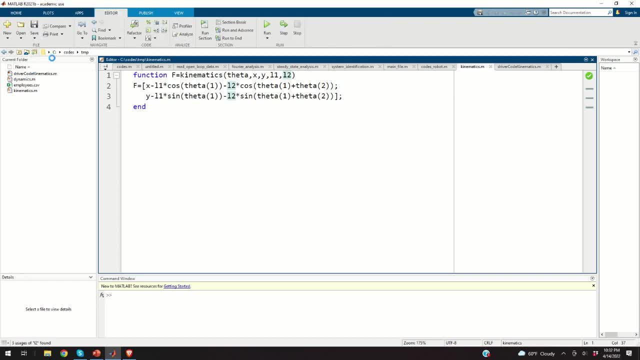 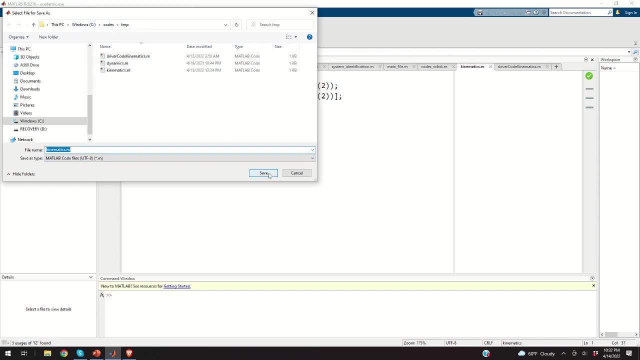 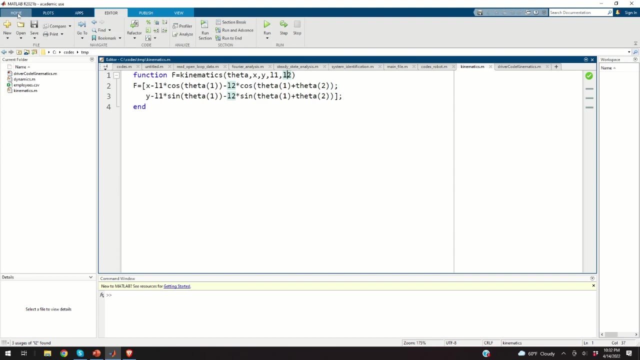 specific file so you can save this function. you click on save as and you can create a folder. in my case it's a temporary folder and I will save this function over here. I will override, because I wrote this script before. the next very important step is to add this folder to the MATLAB path. so you click. 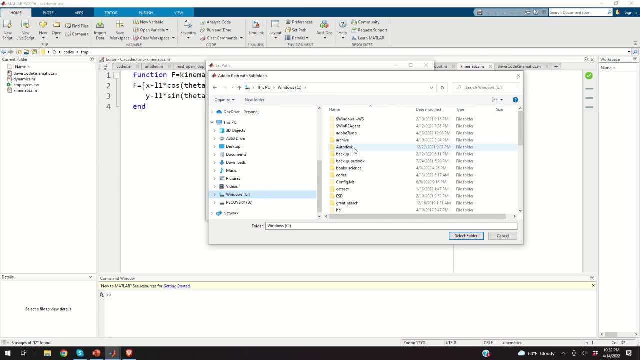 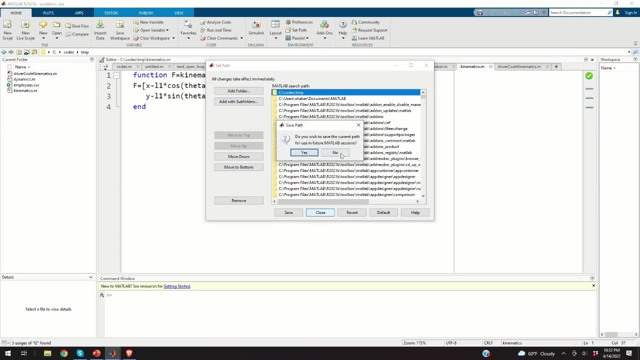 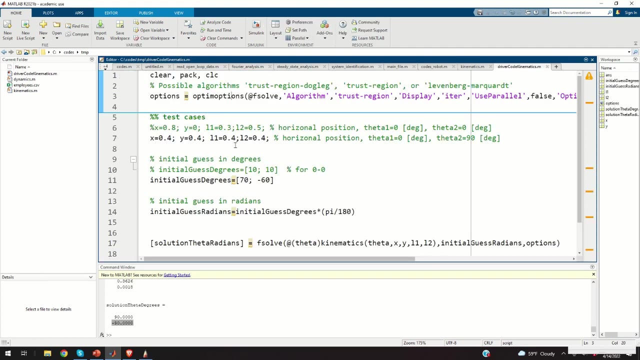 here on add with subfolders, and you need to add the specific folder to your MATLAB path. this is important since we will call this function from another MATLAB script. next, we explain the driver code for solving the system of nonlinear equations. but before we start, I have to mention one very important fact. first of 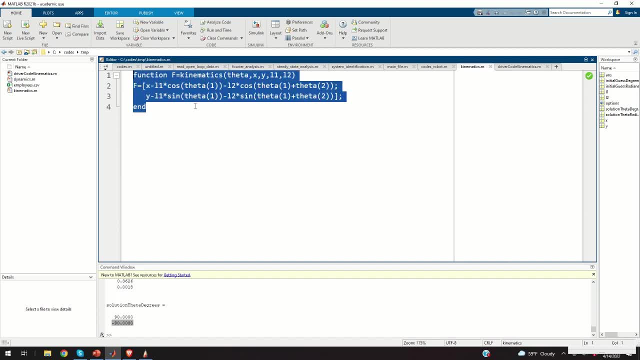 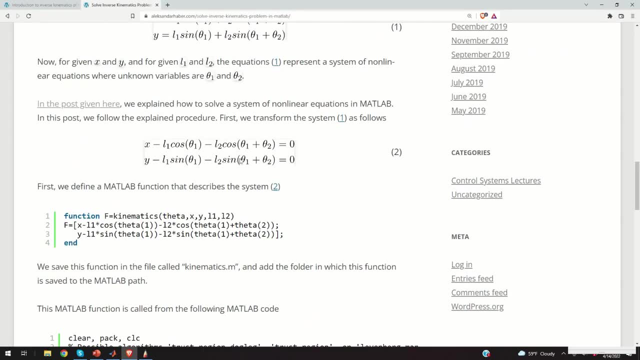 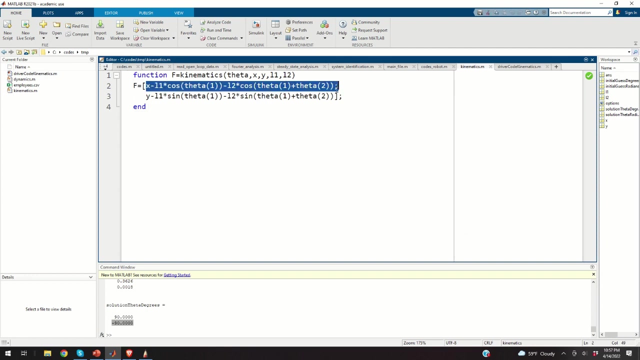 all notice how our system is written in MATLAB. we have basically defined a vector function that gives us the value of our left hand side of our system. so if the solution theta 1 and theta 2 are correct, then the vector f will have very small values. so the first entry. 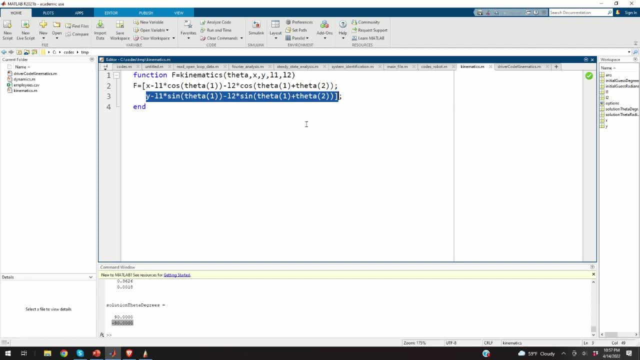 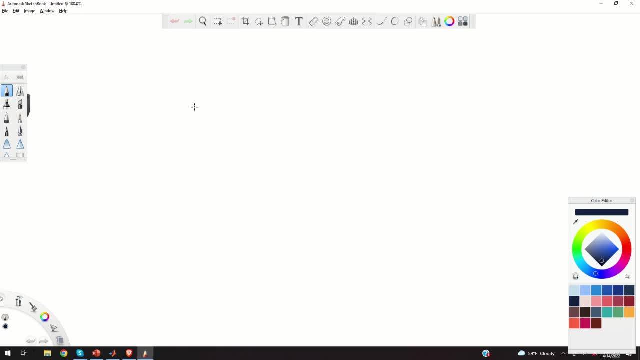 will be very small, and the second entry will be also very small. now, behind the hub, MATLAB is solving the system of nonlinear equations by formulating and solving an optimization problem that has a form that's very similar to the form that I will explain over here. so we have 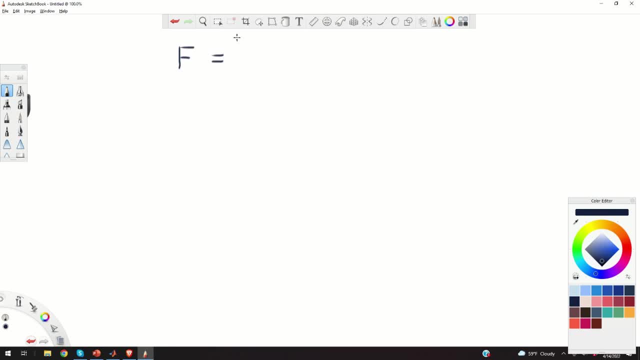 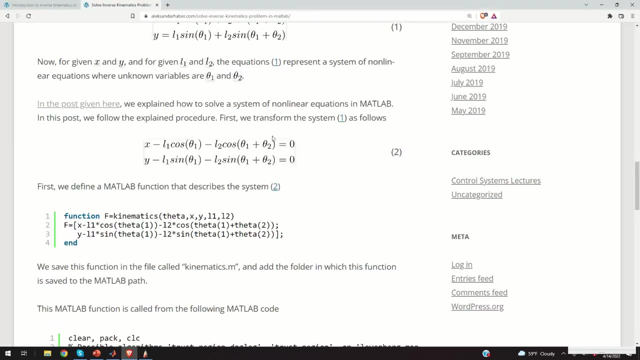 our vector function f, and this vector function has the entries f1 and f2. these f1s and f2s are basically the equations in this system. so f1 will be left hand side over here in the first equation and f2 is in the second egg on the right side of the ε. f1 the first equation and f2 is in the first equation. so this is very easy to train. enter f1 and f2 and data. we have to find the Bakers and you should remember that a vector f is rather common text of the family variable. so we will only be restrained on f2 and some other variables. so this will always be valid in f1. 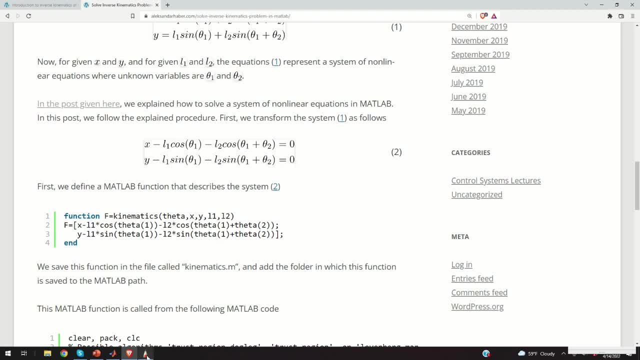 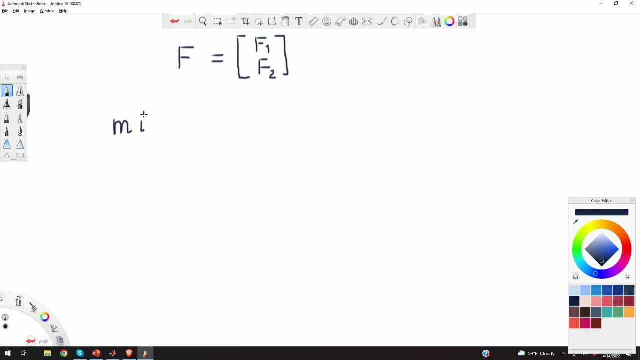 and f2 will be left-hand side over here. the second equation Now. MATLAB aims at actually solving this optimization problem: Minimize, with respect to Theta, where Theta is a vector consisting of Theta1 and Theta2, this objective function. So this objective function is Euclidean 2-norm. that's being squared, It should. 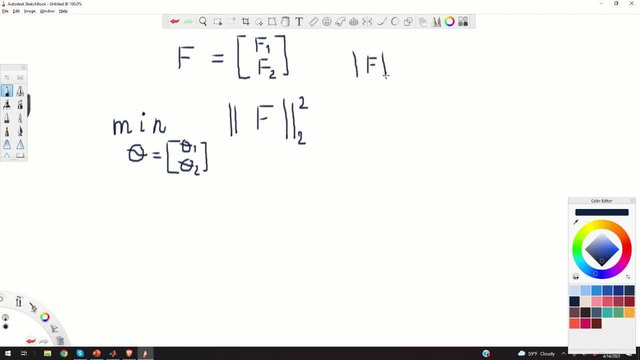 look somehow like this. So, basically, if we expand this cost function, we will obtain something like this: F1 of 5xF0 square plus f2 square. Now you might ask me the following question: Why does this work? Well, if the solution is correct, that is, if theta 1 and theta 2 are close to the solutions. 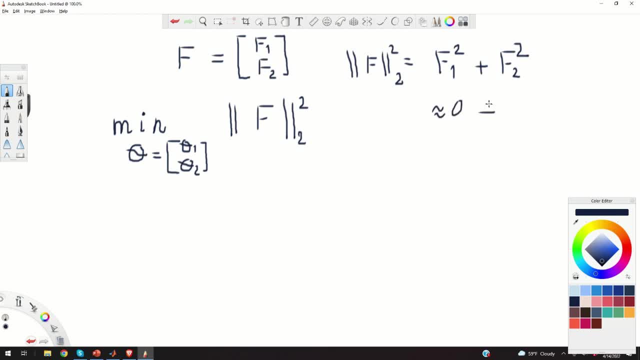 f1 will be close to 0 and f2 will be close to 0. So, basically, if the solutions are correct, our function, our objective function, will be close to 0. So we're trying to minimize this objective function. By minimizing the objective function, we are actually ensuring. 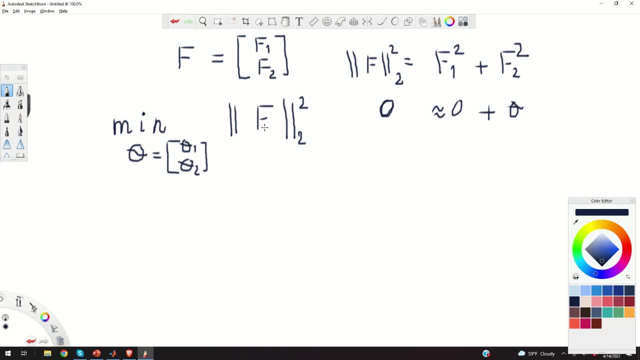 that theta 1 and theta 2 are close to the exact solutions. So this is what is happening behind the scene: MATLAB will try to solve an optimization problem Here. I have to mention that there might be slight variation on this theme, right? So? 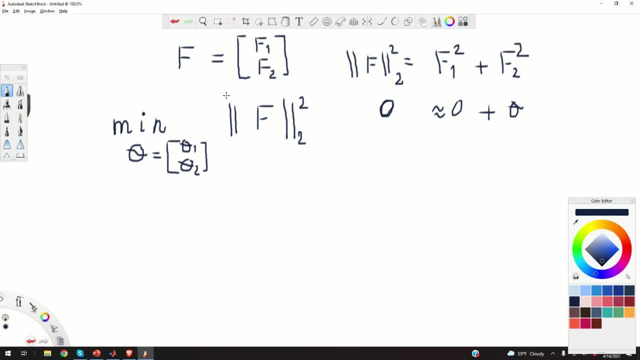 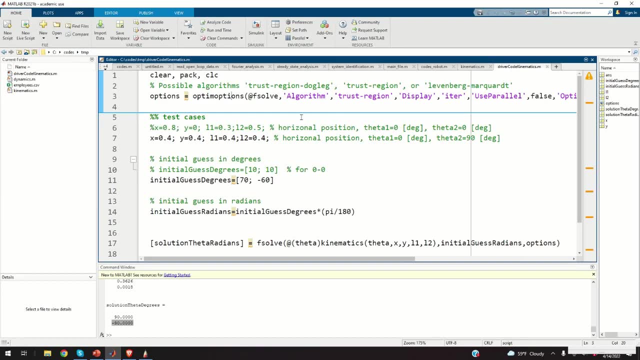 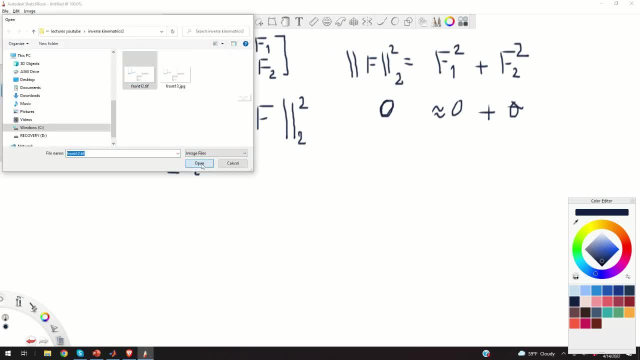 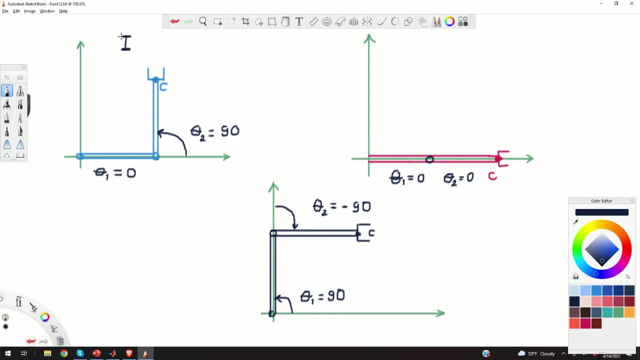 that we have a problem with the algorithm. So let's say that we have a problem with will look physically, from the physical point of view, okay, so this is the test case one, the one that i currently explain here. these are the x and y coordinates: 0.4 and 0.4. so this is. 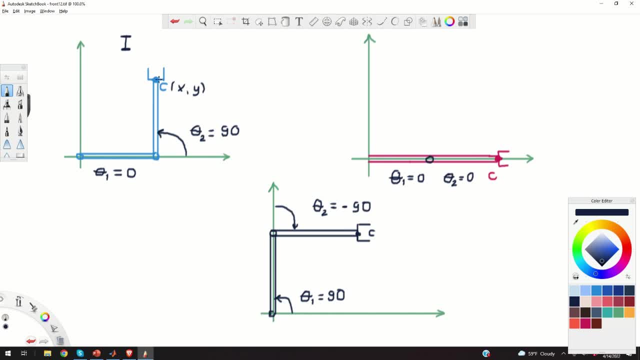 0.4 in x, 0.4 in the y direction. and now from basic graph we can see that basically the true solution should be: theta 1 is equal to 0 and theta 2 is equal to 90 degrees. so we expect that our 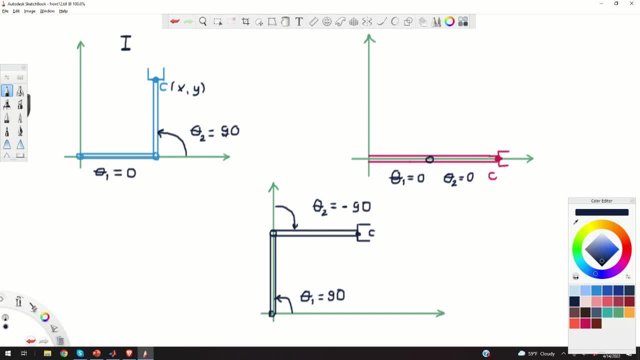 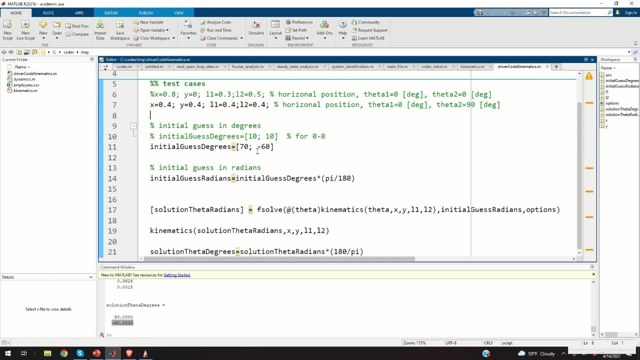 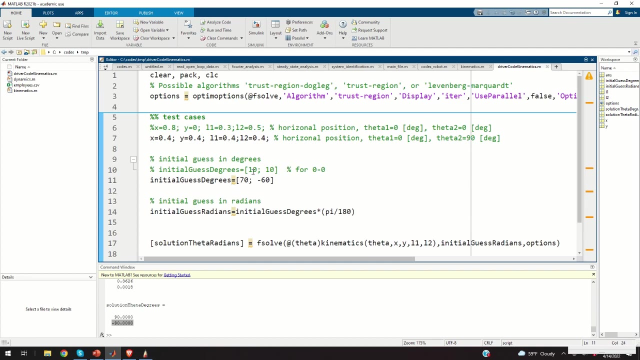 procedure will give us theta 1: 0. theta 2 is 90 if we specify this position. okay, so in order to basically run our algorithm, we need to specify the initial guess for the solution, and here you should really keep in mind that your initial guess for theta 1 and 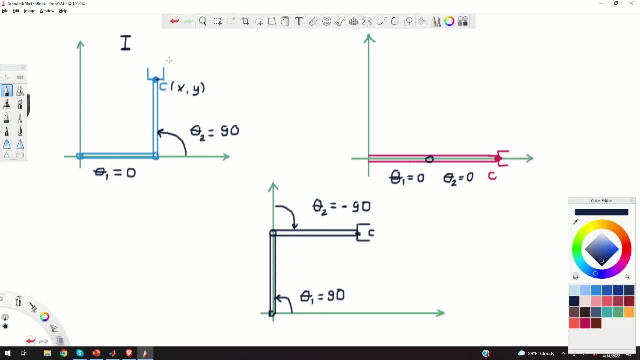 theta 2 is equal to 0 and theta 2 is equal to 90 degrees. so we expect that our procedure will give us theta 1 and theta 2 has to be relatively close to physical configuration. where do you expect that your end effector will be and how the robot will be positioned? what is the configuration over here? 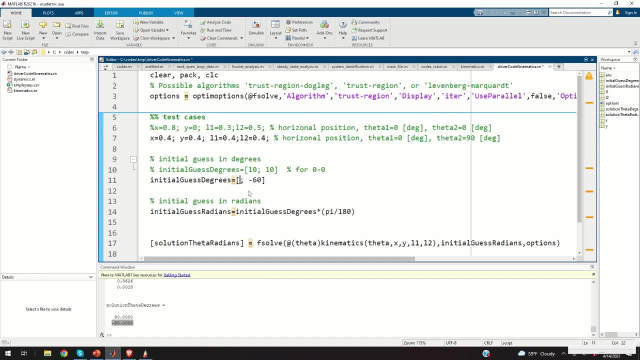 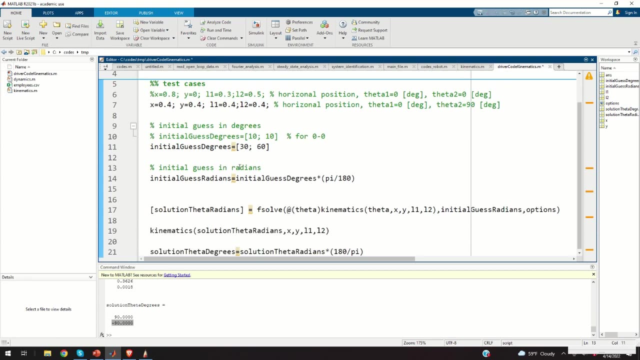 okay. so here i expect, for example, a small value for theta 1 and i expect, let's say, a larger value for theta 2.. so i will use 30 degrees for theta 1 guess and 60 degrees for theta 2 guess. now, since this is initial. 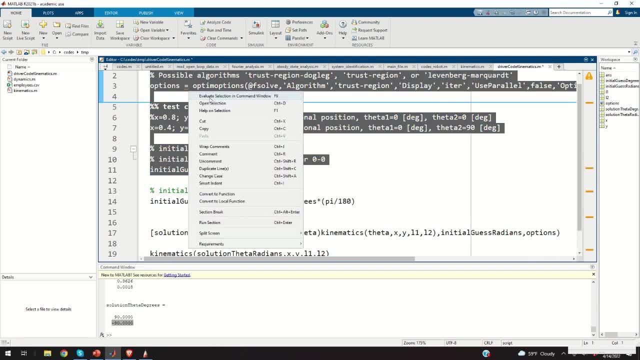 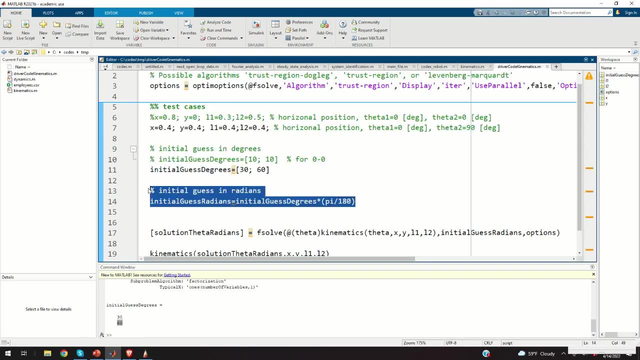 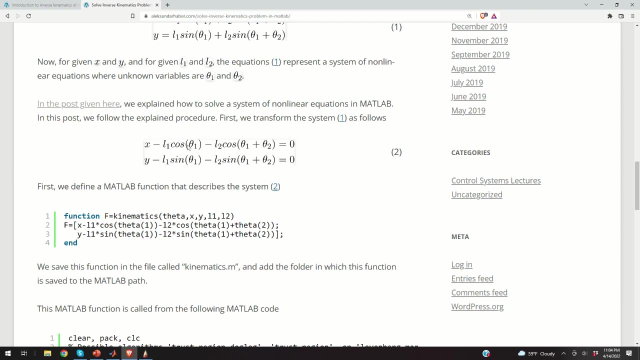 guess in degrees. let's run this, let's see. so here is my initial guess: 30 and 60.. i need to transform everything to radians, so this will be my initial guess in radians. again, you should keep in mind that cosinus function takes radians as arguments, right, although there is a matlab function called 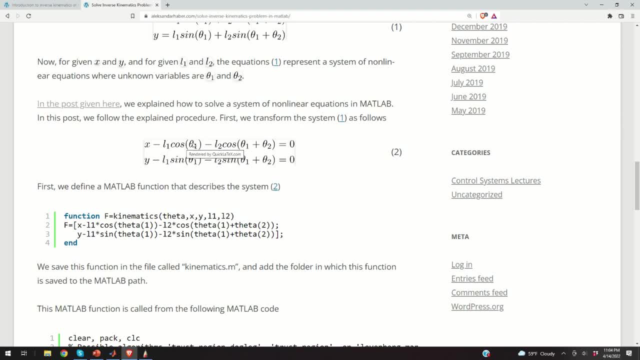 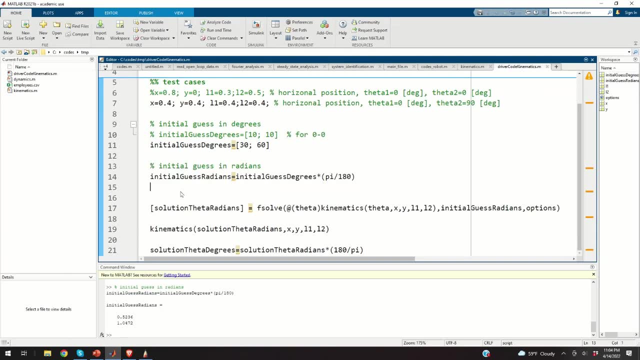 cosinus d, cos d, that takes degrees as arguments. however, this particular function, cosinus, takes radians as arguments. so i need to transform my solution- you know, actually initial guess to radians and over here i will call the function f solve. i will probably call the function f solve. 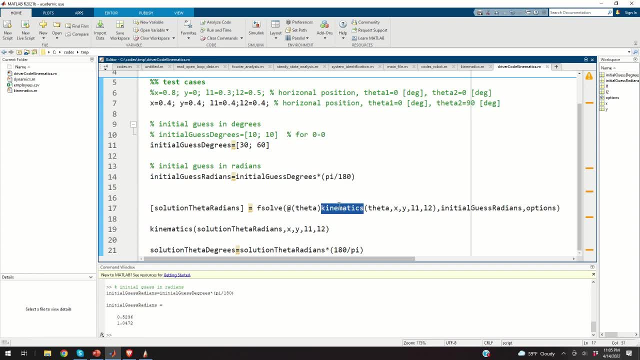 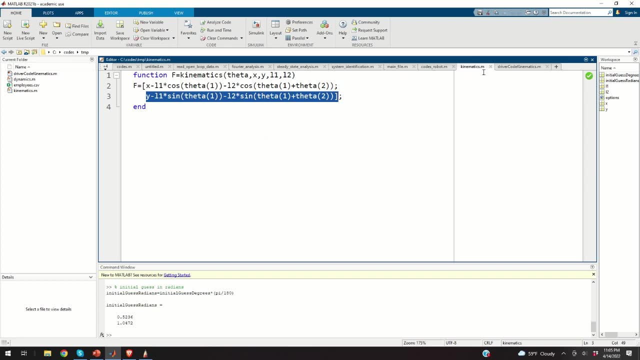 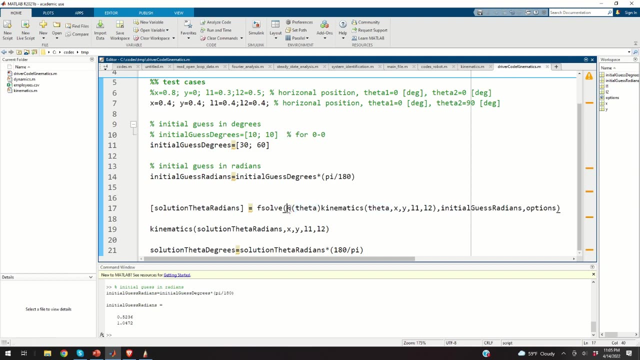 I will provide as an argument my kinematics, the function where I defined my system of nonlinear equations. I need to specify the argument here that this means at theta means that the solution will be evaluated at theta And to this kinematics function I need to specify theta. This will be my basically solution right that will be iterated. 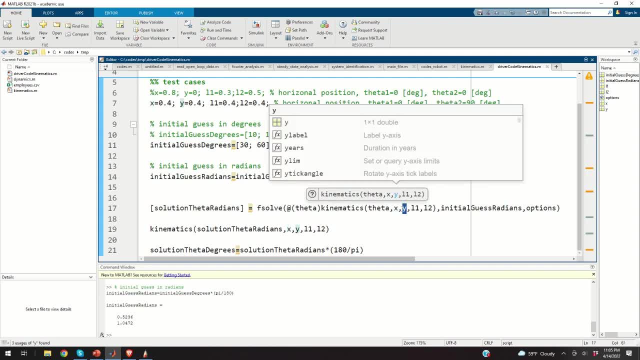 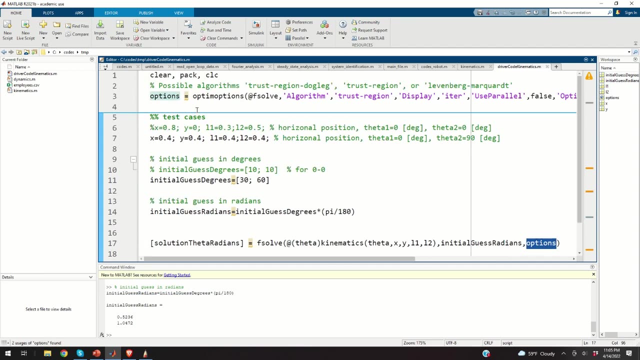 This will be x, y, x and y coordinates that I specified previously, and the lengths of the joints, or actually lengths of the segments. Then I need to specify initial guess in radians and it's very important to link these options To the function, to the fsolve function. 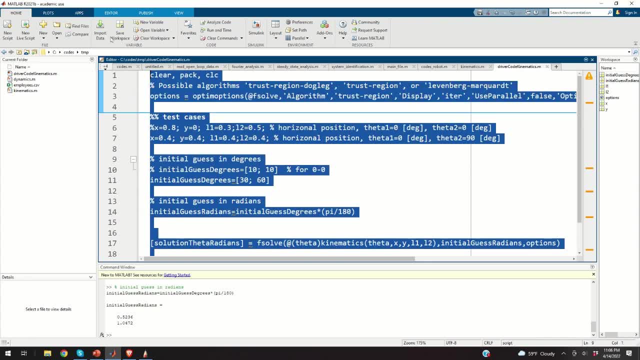 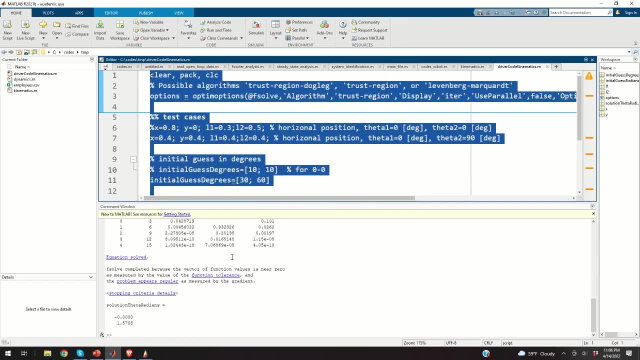 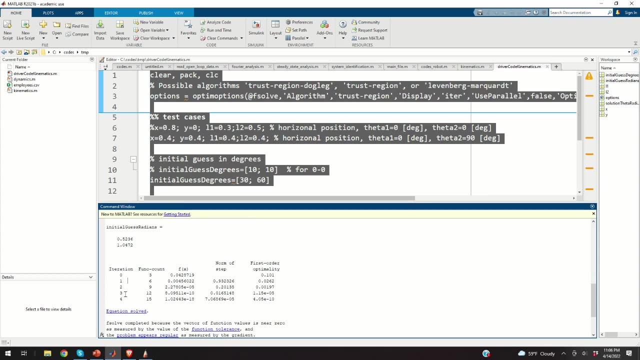 Okay, let us run the solution and let's see what happens. Okay, so here's our diagnostics. We have five iterations. We have how many function counts? 15 function counts. And here's our objective function. Here's our function f. 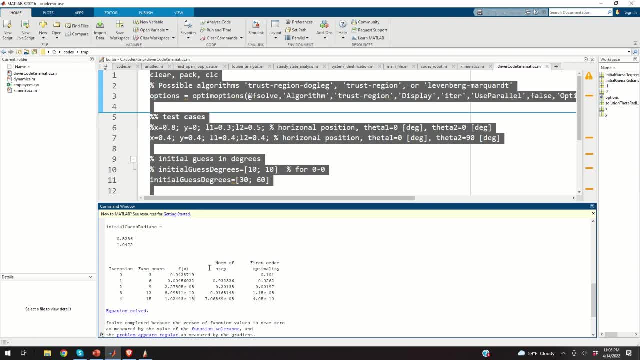 Actually that's defined as Euclidean squared norm of our function f. Here's the norm of the step. Norm of the step is basically Euclidean norm of the optimization step. And here's our optimality. We can see that the equation is solved. it's relatively stringent under stringent tolerances. 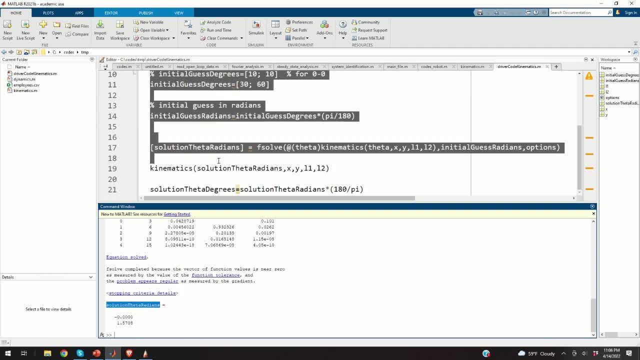 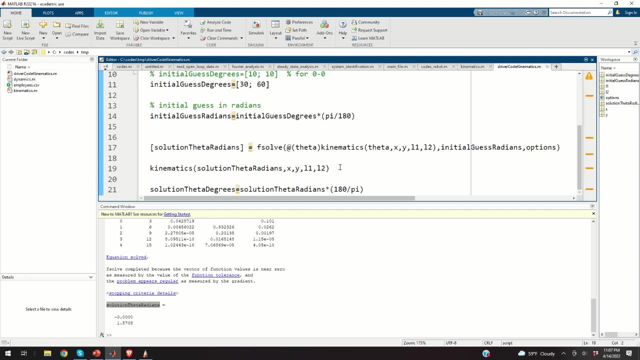 And here's our solutions in radians. Now, before we, Before we convert the solutions, the solution from radians to degrees, it's interesting to analyze the solution. So let us evaluate our solutions in radians And let's see the value of our function f. 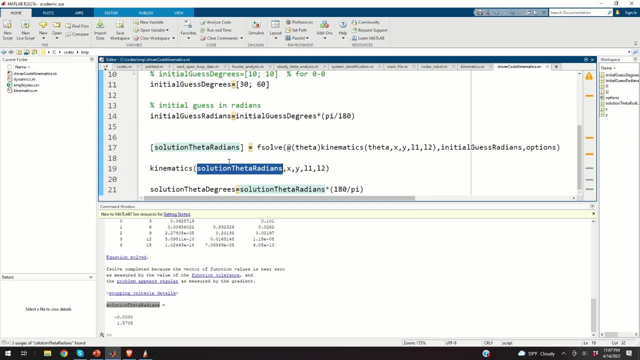 We expect that for basically the solution, the value of the function f will be small. So by calling the kinematics specifying the solution in radians x and y, coordinates l1 and l2, we should just get the value of f, since this function returns f. 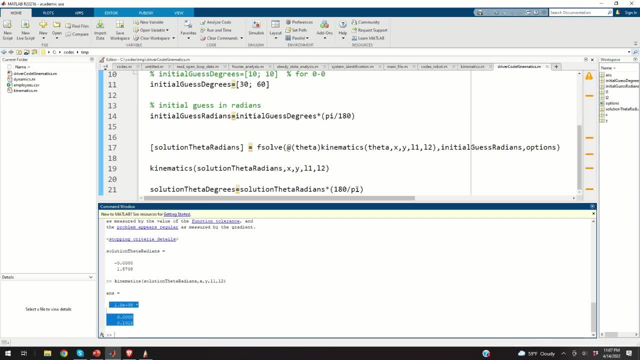 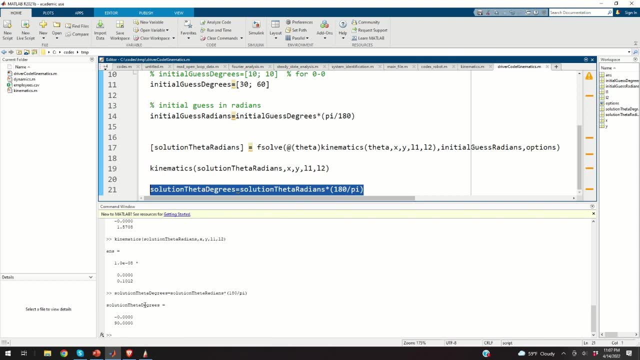 And we can see that f1 is small and f2 is small, So the solution should be okay. Let us convert the solutions to degrees, And voila, here's our solution. Theta 1 is 0,. Theta 2 is 90 degrees. 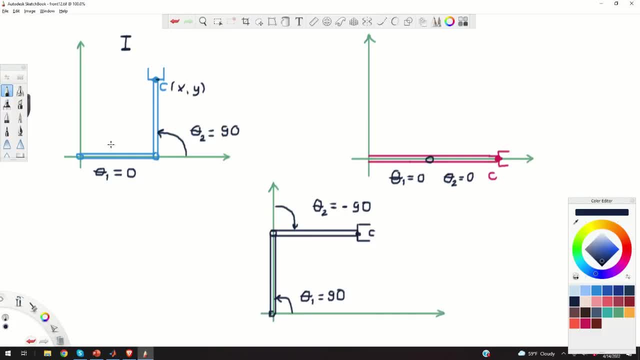 So we're able Actually to find the true solution. This is the test case 1.. In my previous video tutorial I explained that the solution of the inverse kinematics problem is not unique And to test that, we will analyze the second test case. 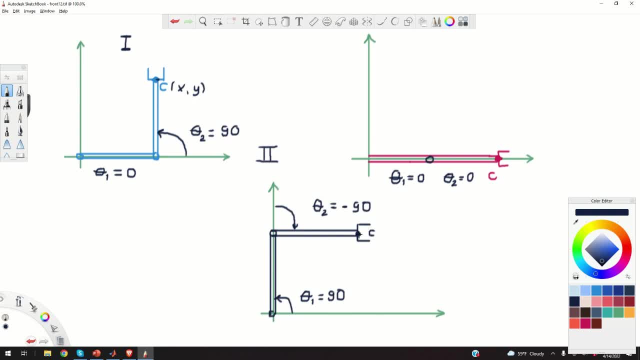 Right. In the second test case, the TCP will be at the same position as in the first case. however, the robot configuration will look differently From physical point of view. we can reach this point either in this way or we can reach it from this side. 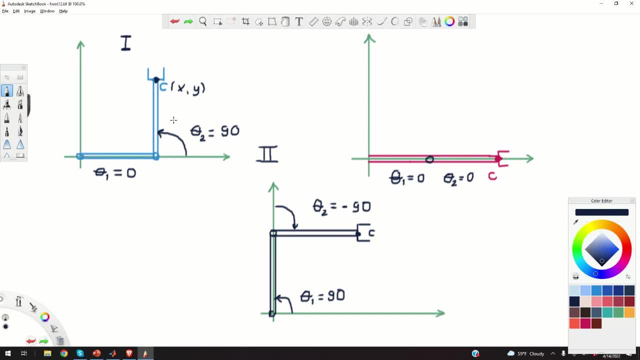 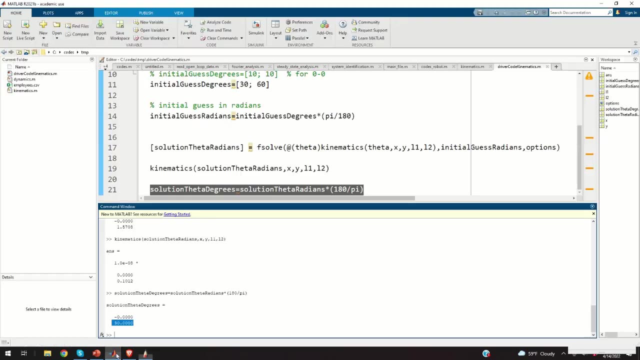 Right. That's why the inverse kinematics problem, or its solution, are not unique, And I explained this in my previous video. So how are we going to test this scenario? Well, to find the solution, in this case, we'll just change the initial guess. 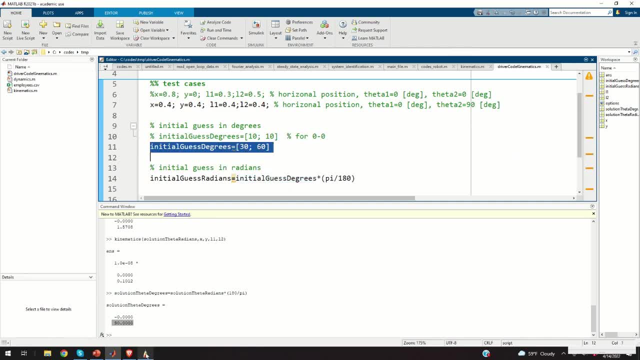 Here, instead of using 30 and 60, we will use a different initial guess. So we'll say that, basically, Theta 1 is around 70 degrees And Theta 2 is minus 70 degrees. Okay, So, by setting the initial guess, 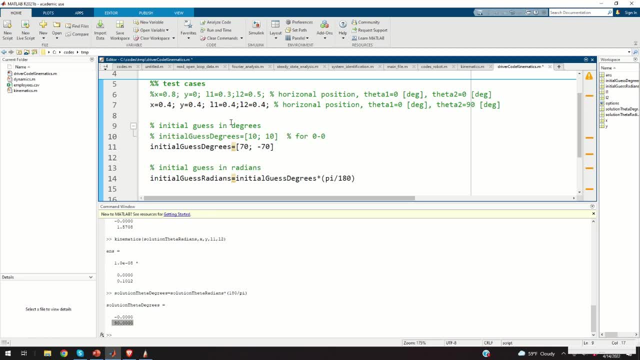 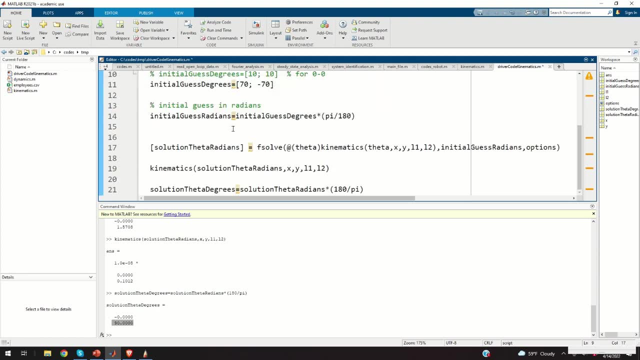 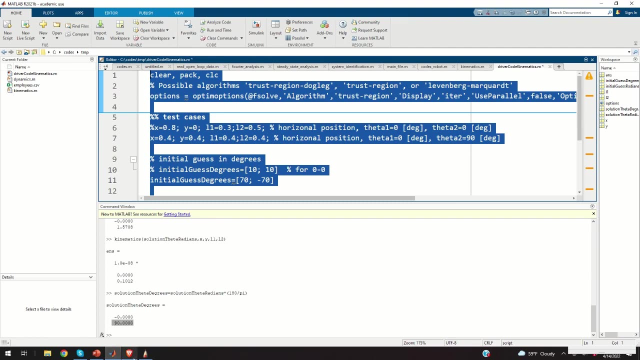 we can actually retrieve different solutions of the inverse kinematics problem, But you need to know what is actually happening behind the scenes. Okay, So let us run the procedure again from the scratch and let's see what happens. We expect that the solution again will be 90 degrees and minus 90 degrees. 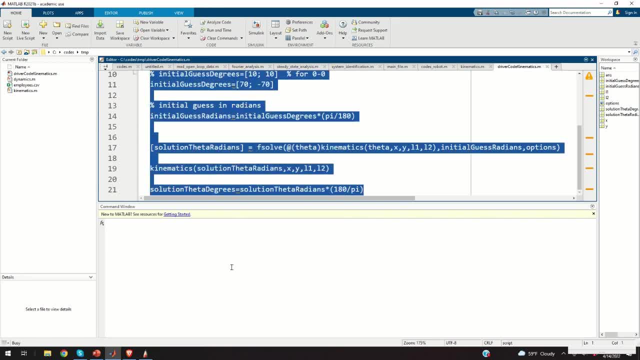 So let's see the performance. Here it is: We are able to accurately solve or accurately compute the solution of the inverse kinematics problem. for the second test case: Theta 1, 90.. Theta 2, minus 90 degrees: Very good.